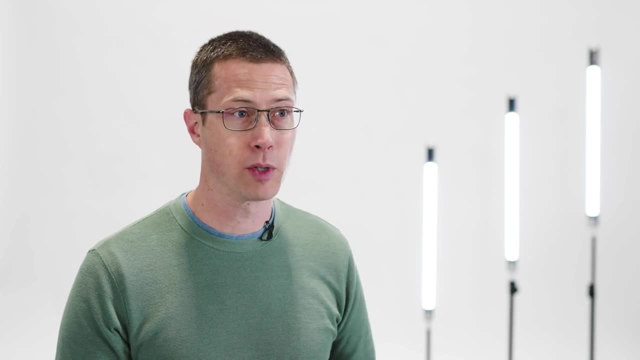 Atrius Early on trying to really capture the dynamics of how animals walk and run. we first looked at the dynamics of how animals walk and run And we looked at the dynamics of how animals walk and run And we looked at biomechanics And we looked to basic math models. 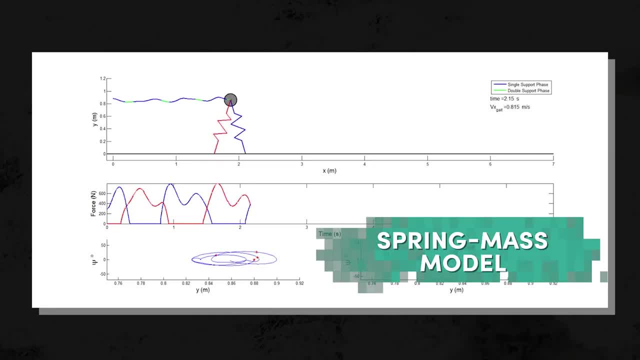 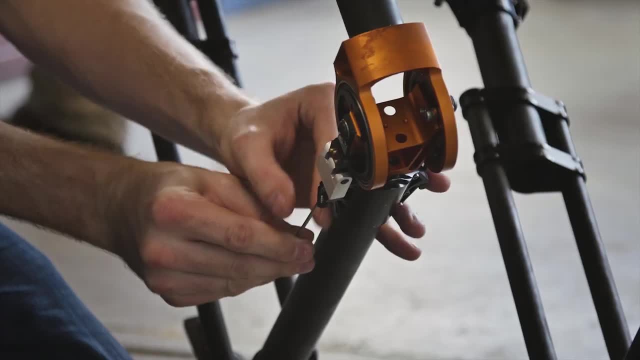 of how do animals walk and run, And we see things like the spring mass model. We set out to build Atrius, which is a machine that is a spring mass model as close as we can get to it. The whole idea was build a machine that's as close to this model as possible and then write really simple controllers. 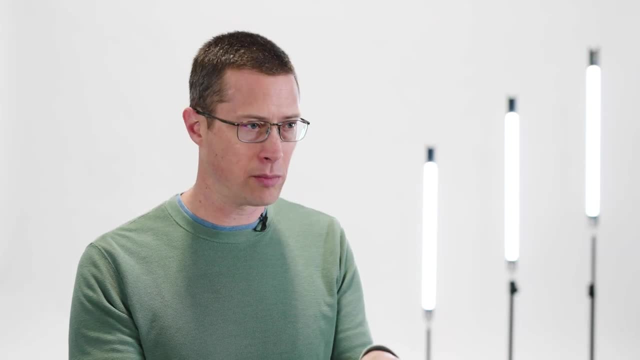 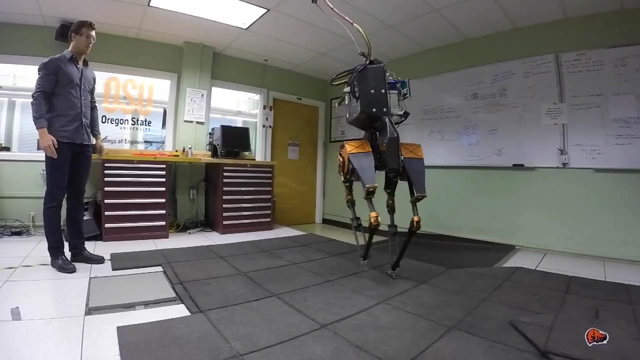 as if they were operating on this simple model. Just apply them to the robot and see if we can get it to really work well. Atrius was a success. It could walk and run over uneven and unsteady terrain And it was the first bipedal robot. 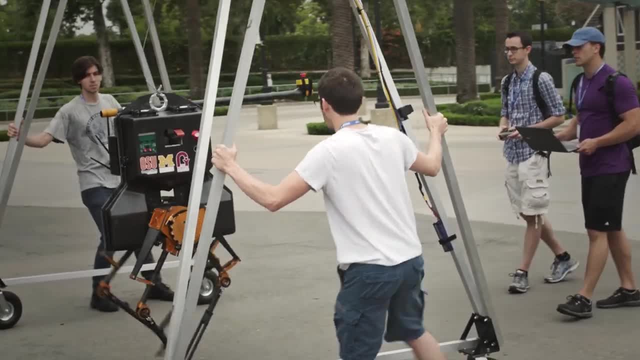 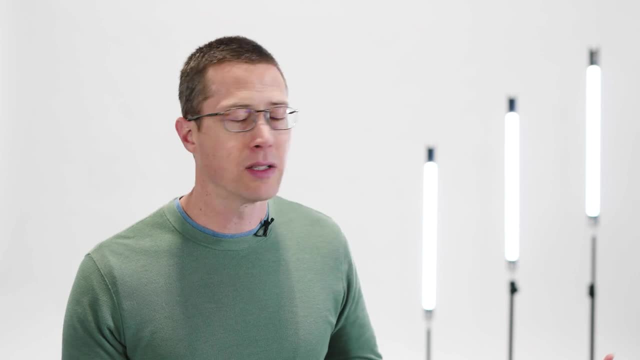 to reproduce the dynamics of the human walking gait. And it did all this without visual perception sensors. But it had many limitations. It was a great science demonstrator, right, But there's all kinds of things wrong with it. First of all, it can't actually stand. It can only. 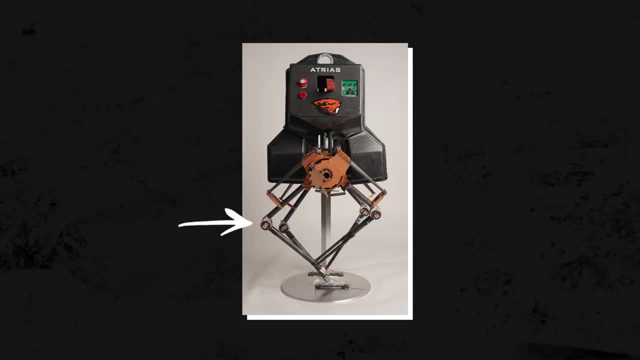 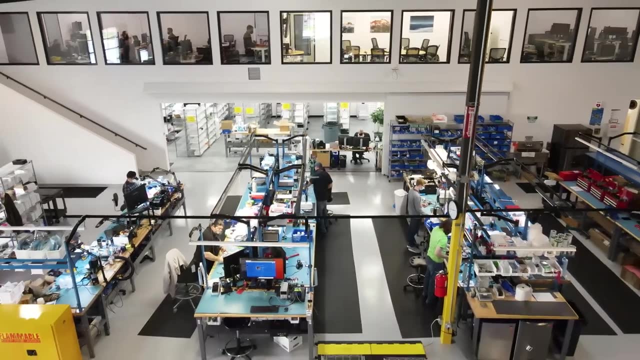 walk and run. It can't turn. This four-bar linkage is like having two knees. It's really not practical. if you wanted to make a robot that goes where people go, By this time Agility Robotics had spun off from the OSU lab into a private company And it was time to apply. 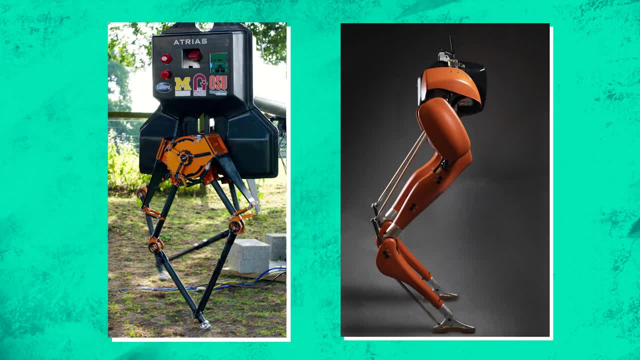 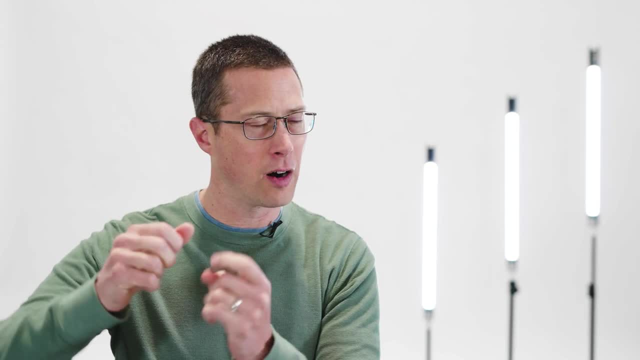 this knowledge into a commercial product. If you really look closely at the CASI design, there's kind of shadows of the Atrius design. Just maybe move one of those linkages really far in and really close and you start to get what looks a lot like the CASI leg. At that point you know it looks like a bird leg. 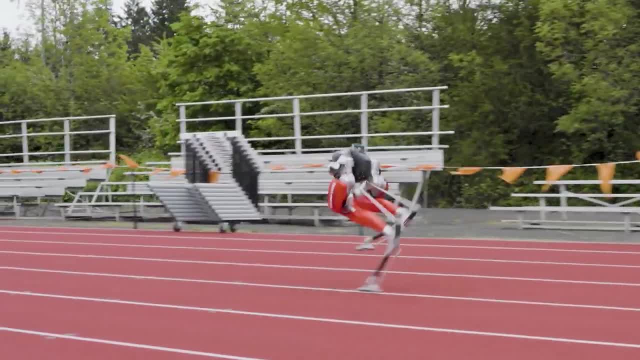 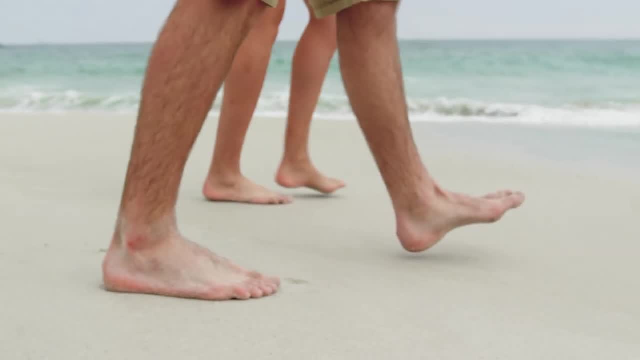 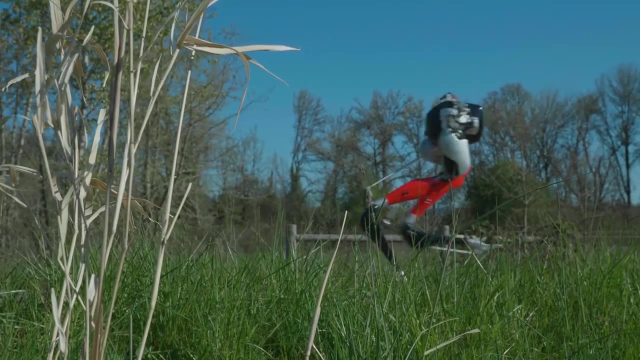 But we certainly didn't set out to make it look like a bird leg. Birds are what's known as digitigrades. They walk and run on their toes as opposed to flat feet like humans. It's hard to make a one-to-one comparison between animals and robots, or muscles and actuators, but the similarities. 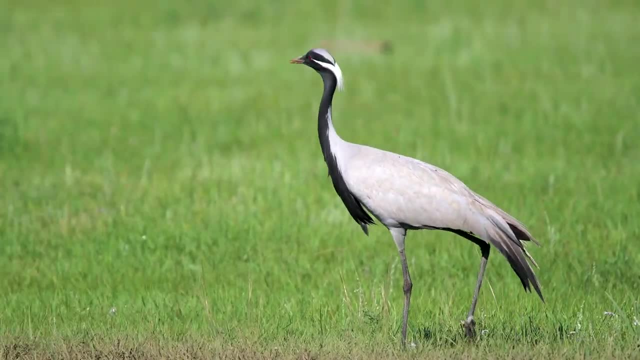 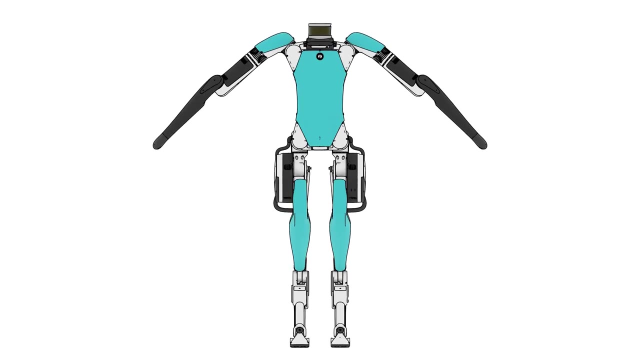 between CASI's legs and a bird's are undeniable. Those similarities were passed on to Digit. Digit built off of CASI's legs, adding a torso and manipulators, And unlike Atrius and CASI, which were effectively blind Digit.